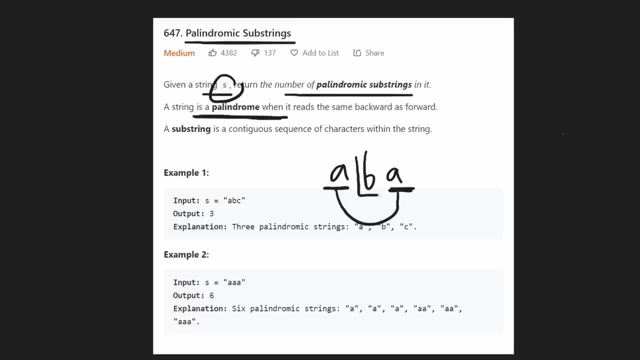 is the same as the last character, And then in the middle we're just left with one character, And you know, basically that kind of pushes us towards a base case. So, as you may know, there's two types of palindromic substrings: strings of odd length, right? So, for example, 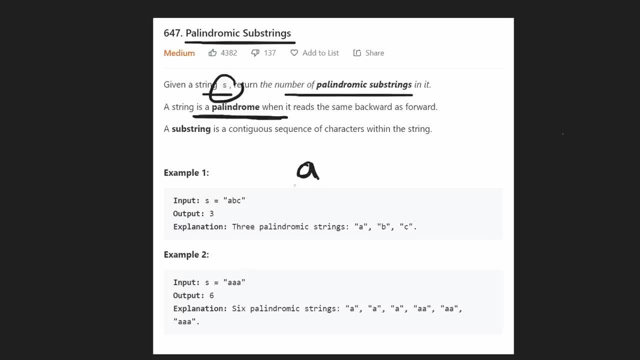 just a single letter A. that's a palindrome, right? It's the same backwards. If we add a B to the beginning and a B to the end, it's still a palindrome. We expanded it outwards with the exact same character. Similarly, we can do the same thing. 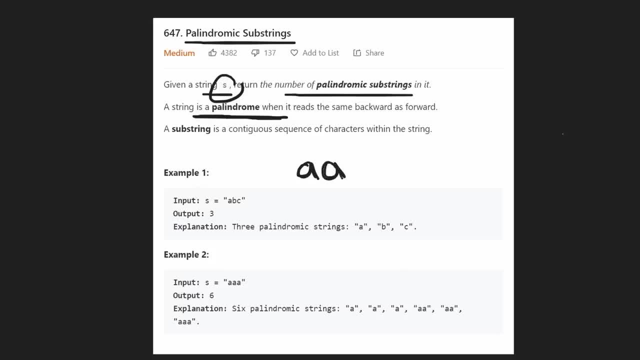 with even length substrings as well. If we have two A's in the middle, then of course this is a palindrome. And then if we continue to expand outwards, we add a B at the beginning and we add a B at the end. it's continuously going to be a palindrome, because these characters are also 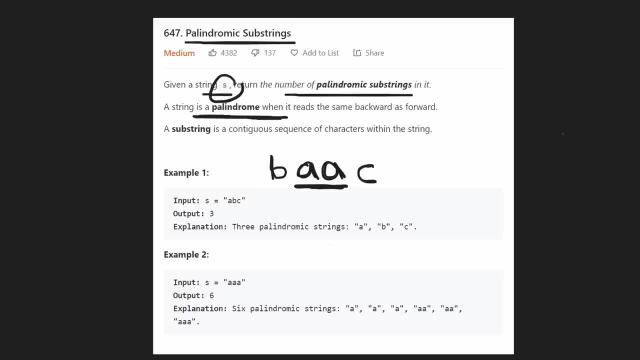 matching. Now if we, instead of adding a B, we added a C at the end, the inside is a palindrome, this string of length two. But now if we expand outwards, this is not a palindrome, right? Yeah, this just it can't be read backwards. C is not. 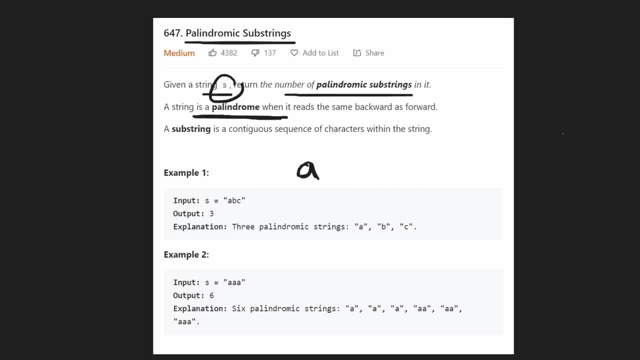 the same as B, it's not a palindrome. So that's a little bit about palindromes, even an odd length. But so how can we apply that to our input? So in this case we are given a string- A, B, C- Now 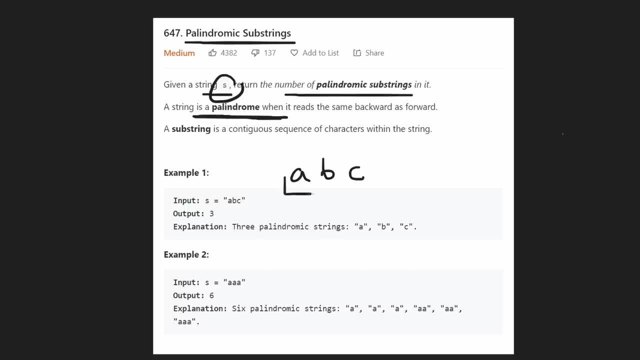 of course we have three different palindromes, because each character by itself is a substring, of course, and each of those by themselves is a palindrome as well. So that's three. Now is any other substring, for example A? 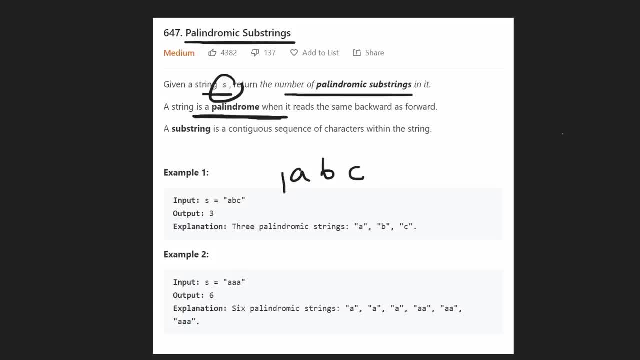 B- that's not a palindrome. B C- that's not a palindrome. A, B, C- that's also not a palindrome. That's basically all the substrings available to us. So we only find three, so we're going to return. 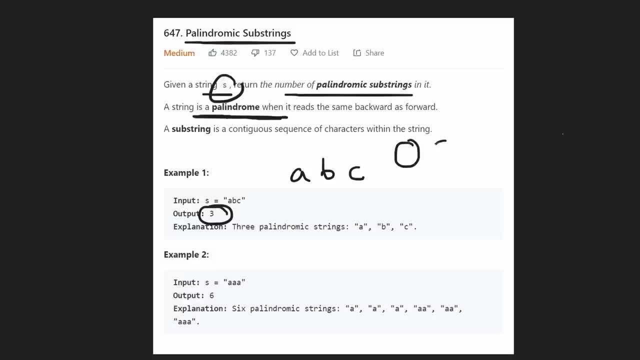 three. So let's understand how we can do the brute force solution, which is actually big O of n cubed, And then we can actually optimize it a little bit, understanding how even and odd palindromes work, And then we can get a big O of n squared time complexity solution. 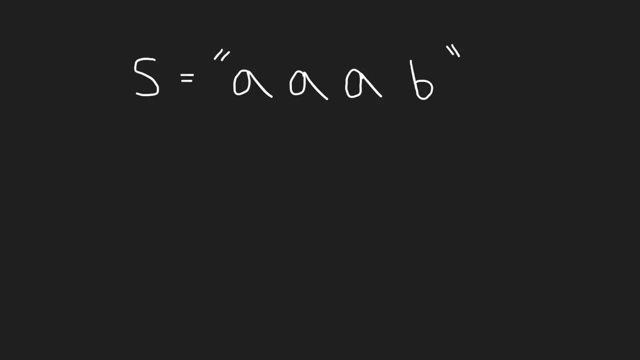 So let's say, we're given a string that looks like this: If we just start brute forcing it, we want to go through every single substring, right. So every single substring starting at this first position would be something like this: right, There's. 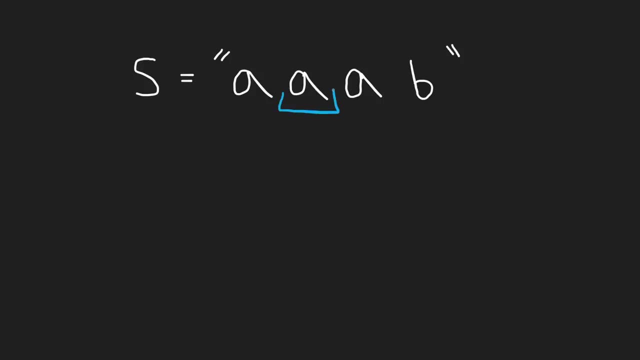 these substrings right. Then we'd want to go through every single substring, starting at this position, which would look something like this: right, In total, there's going to be n squared substrings, right, And for each substring, for example, you know, this one we need to determine. 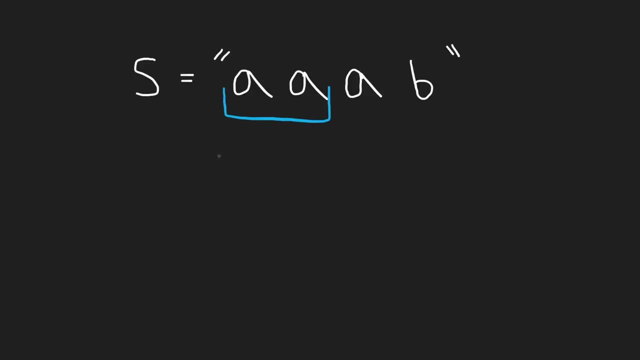 if it's a palindrome or not, And we know, you know, that's not a difficult algorithm, right? We could have two pointers: one at the beginning, one at the end. We basically keep comparing the characters and making sure that they're the same right? So, and for a substring, 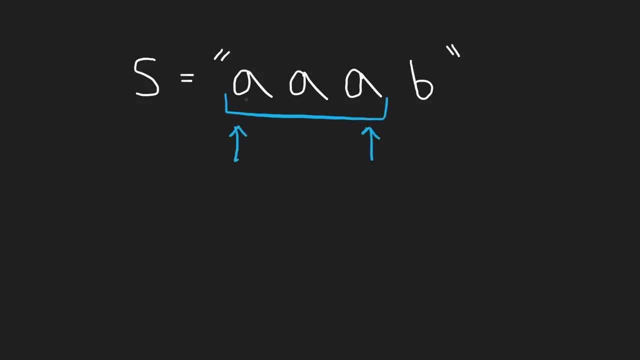 like this: we'd also have two pointers, right, Compare that, okay, these two characters are the same. So then we can move inward, right, We'd shift our pointers here and then we'd see, okay, this character is also the same. And then, you know, we go through every character, So we 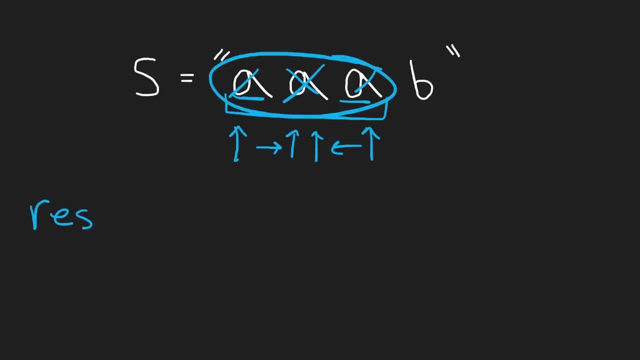 determine- yes, that's a palindrome- Then we can increment our count of palindromes, right, We'll call that our result variable. So then what we're going to do is we're going to go through every palindrome and we're going to add one to it, right, Because that's ultimately what we're. 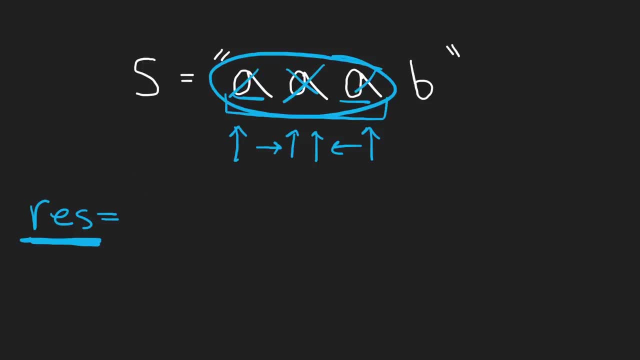 trying to return the number of palindromic substrings inside of this string S And clearly, finding and determining that a string is a palindrome is also big O of N. So since there are N squared substrings in the entire string S and for each of those substrings we have to 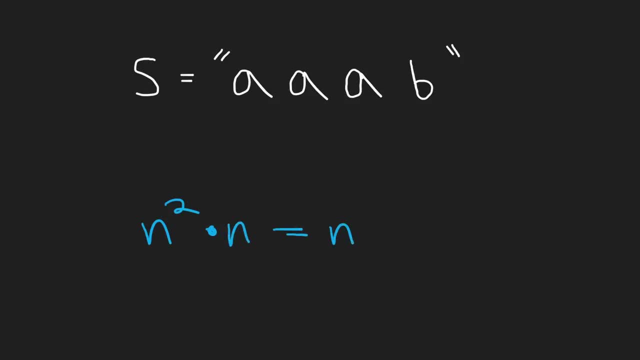 determine that it's a palindrome, We're going to multiply it by N, So this is going to give us an N cubed time complexity. Now we can improve this, and it's going to require us to solve this problem in a different order. What we're instead going to do is we're going to go through. 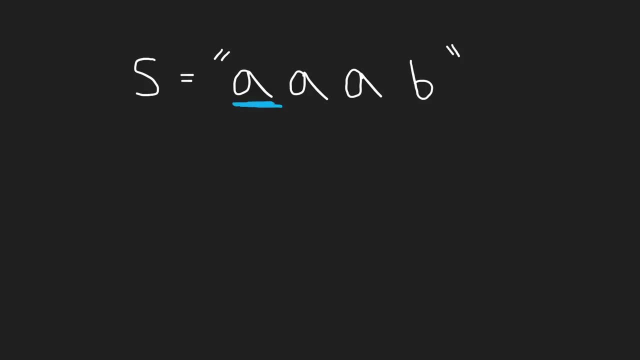 every single position in this right. Instead of finding, for this position, all the substrings that start at this position, we're going to find all the substrings that this position is the middle of. So instead of, you know, just going to the right, we're actually going to expand in both. 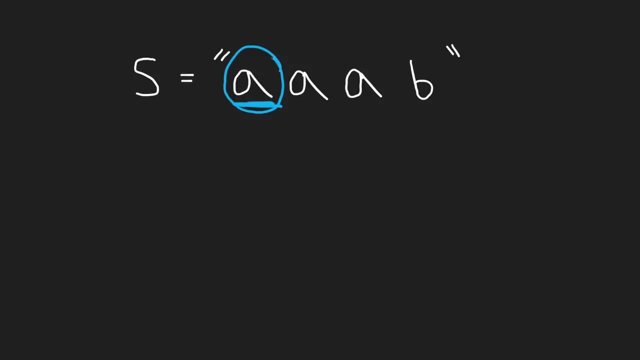 directions. We're going to go through all substrings where this position is the middle position. Now, clearly, this string itself is a palindrome, So we're going to find all the substrings where this position is the middle position. So, instead of finding all the substrings where this 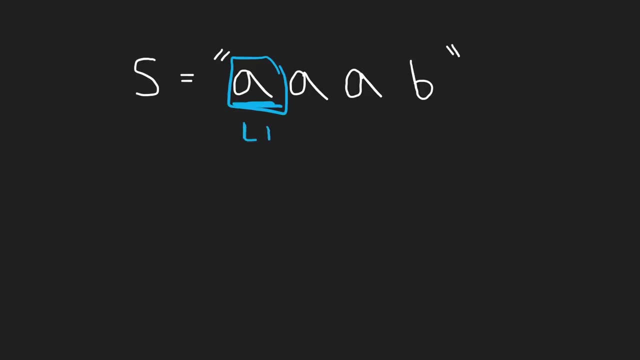 position is the middle position. Now, clearly, this string itself is a palindrome, So we're going to have our left and right pointer just initially at this position. We're going to see that, okay, both of these characters are the same, right? So then we can take our result, add one to it. 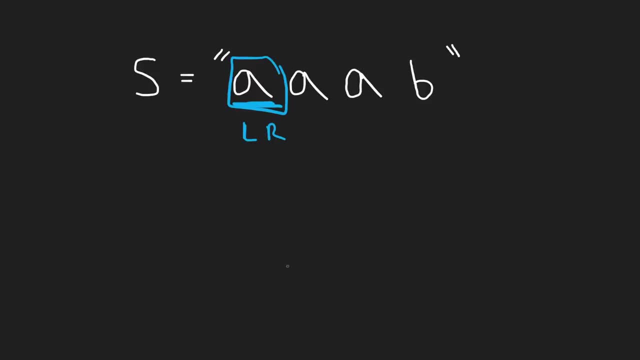 right. So we found- so we did find- one palindromic substring, and then we're going to try to expand outward right. Our left pointer is going to go here, Our right pointer is going to go here. Clearly, we go out of bounds, though, to the left right. So so, basically, what we're saying is: 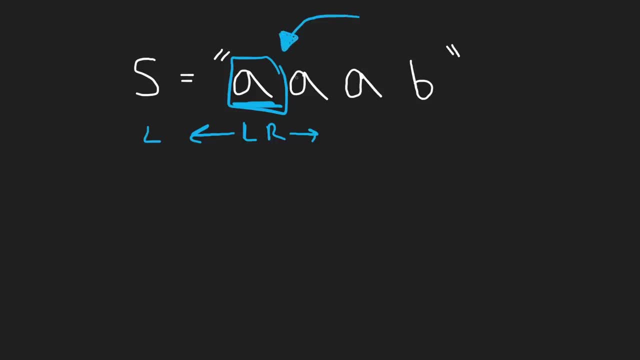 there's only one substring where this is the middle position of, and then we're going to do the same for here. So from this position, we want all substrings where this is the middle of. So we're going to have our left and right pointer initially here. Yes, this character, you know our left and. 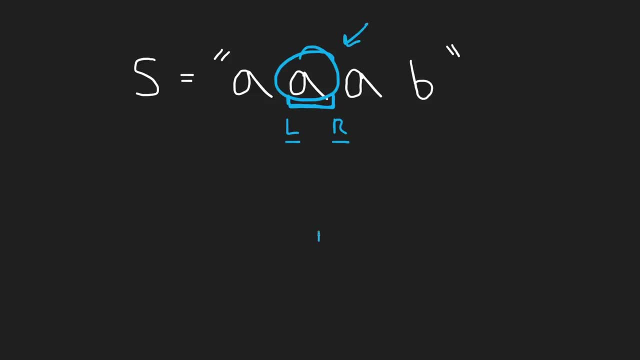 right pointer point at the same character. So we we found one palindromic substring, just the single character itself. Then we are going to take our left and right pointers and then shift them. So left is going to go over here, Right is going to go over here right. So now let's compare left. 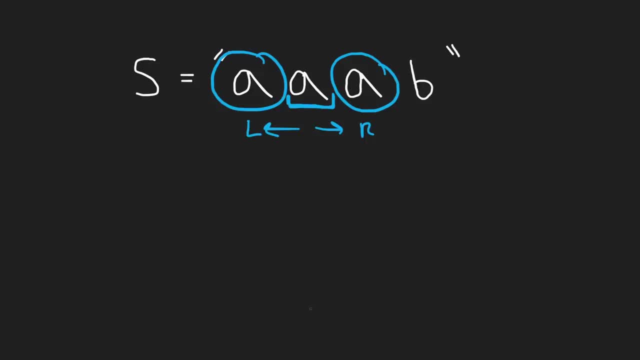 character and right character. Since, we already know, this middle portion is a palindrome, right Now we only have to compare the left and right characters, the new left and right characters, if they are equal right, Which they are, a equals a right. So therefore, we found one additional. 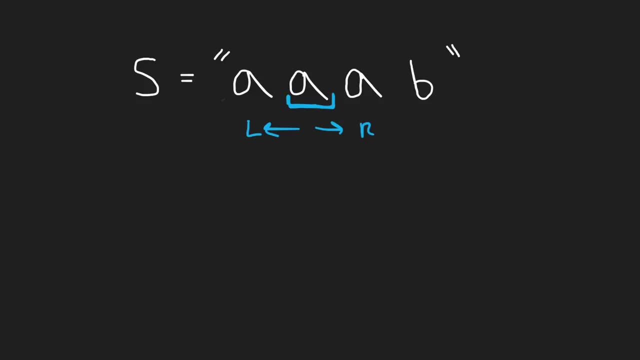 palindrome, this palindrome of length three, where this character is still the middle position right. So now we found an additional palindrome, So I think our total number of palindromes is up to three now And once again we're going to take our left pointer, shift it to their left. 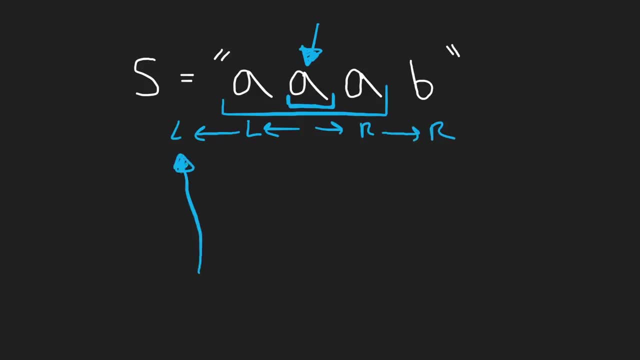 right pointer and shift it. Now clearly, once again, our left pointer goes out of bounds. So you know, this is- we can't really find any more substrings- where this is the middle position. But do you notice how, what we just did, right, We we cut down on repeated work. We found that. 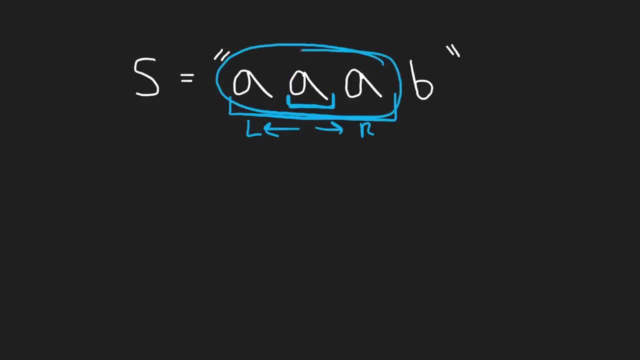 this is a substring. And then in another single operation we found that this is a palindromic substring as well. That cuts down on the repeated work, Whereas before we would have done something like: okay, you know, this is a palindromic substring, Then we increase it. 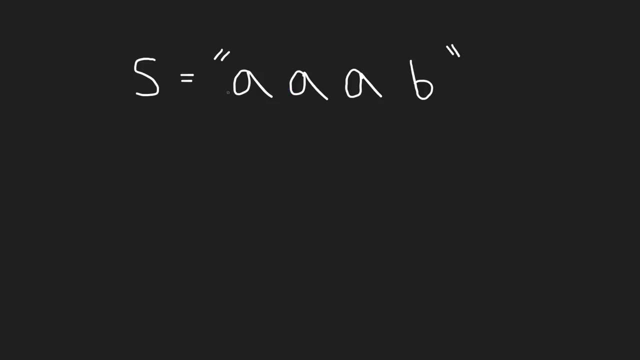 Then we have to look at both of these. And you know, if we continue to increase it, if we go all the way here, then we have to still check. okay, this is the same. And now, this is the same right. 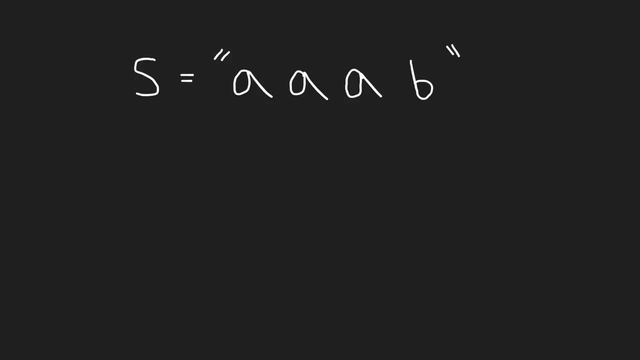 We're continuing to do repeated work if we start from the left and then expand to the right, But if we start in the middle and expand left and right, then we eliminate repeated work. So let's do the same thing from here. So this is a palindromic substring: right, Left and right. 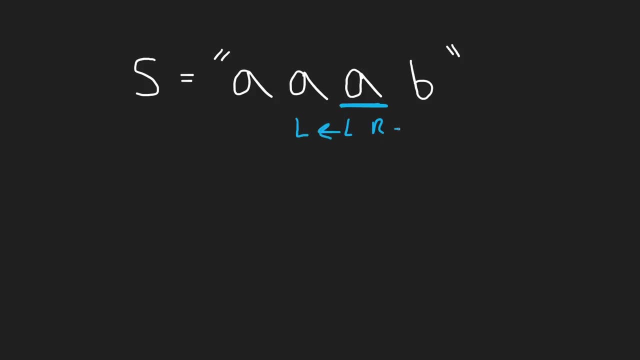 point at the same character. Then we expand once to the left, once to the right. are these characters the same right? Are A and B the same? They're not the same. So we knew that the initial substring, just in the middle over here, the single character, was a palindrome. 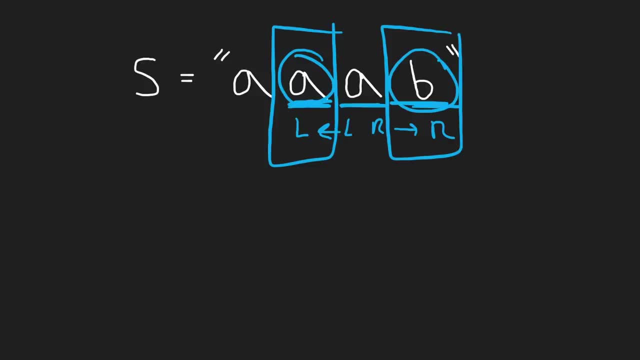 But when we add this character and this character, it's no longer a palindrome. This is not a palindrome. So, no matter what we do now, if I expand one more to the left and expand one more to the right, even if these characters were the same, assume we had an A in both positions. 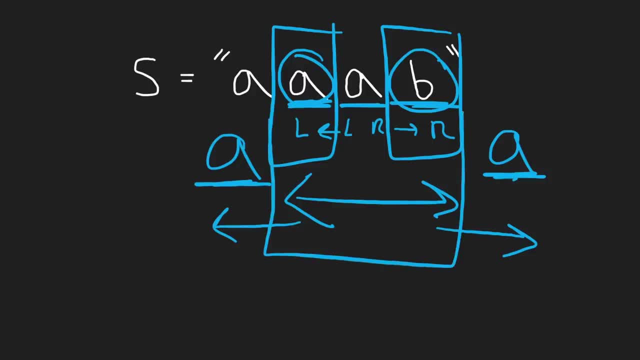 because the substring in the middle is not a palindrome. So therefore, no more substrings expanded from the middle of this position to the left and right. None of those additional substrings are going to be palindromes. So so far, our count of palindromes is at four. 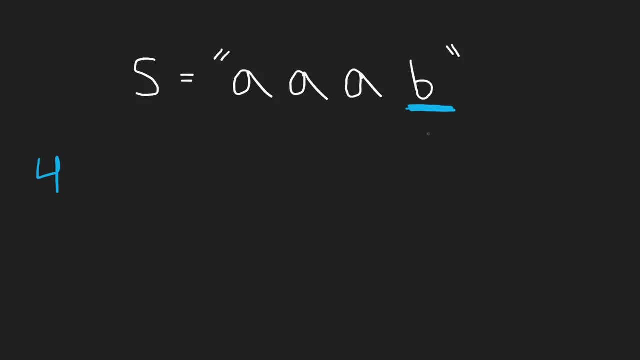 I believe. So now let's go to the last position. So we want to expand from this middle position. So initially we're going to say, okay, this itself is a palindrome, So we can change our count of palindromes to five. We try to expand left and we try to expand right, But again, 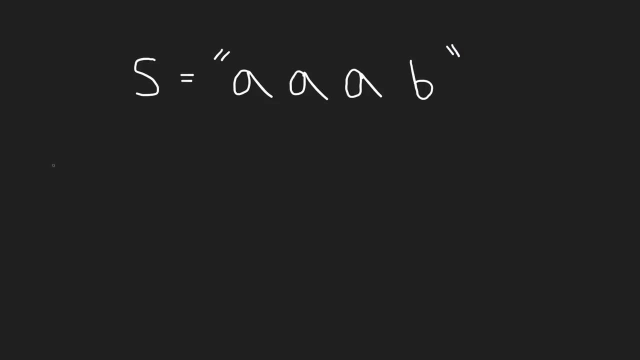 we go out of bounds to the right side, So we're done. So in total, we found five different palindromes, but it turns out we actually missed a couple. We missed this palindrome of length two and we missed this palindrome of length two. How is it that we missed palindromes And how is it? 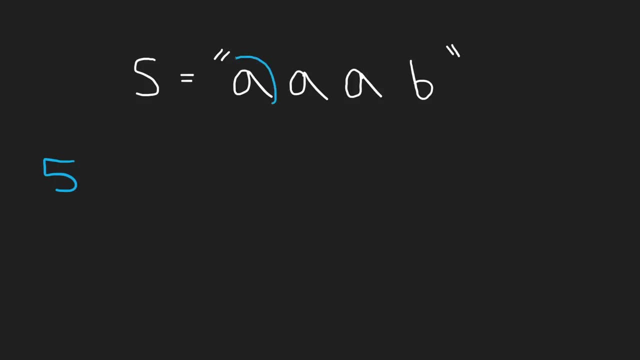 that they're both length two. Notice how we were starting at each middle position. So this was a long time ago. So we're going to expand left and we try to expand right, But again we go out of bounds to the length of one right. As we add the adjacent positions, then we're increasing. 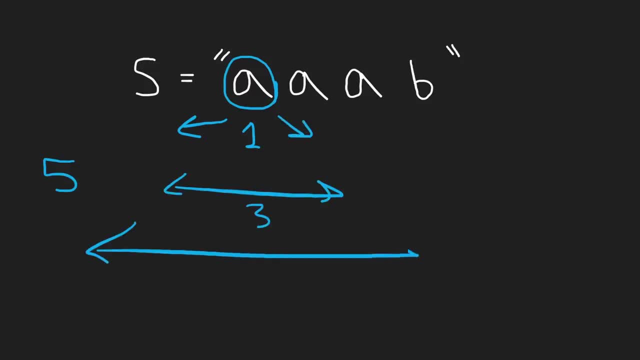 the palindrome to length three And then, if we added a couple more, we'd increase it to length five. So we're only getting palindromes of odd length. If we want to get palindromes of even length, we have to start at every single even position. So we'd have to start at here And then 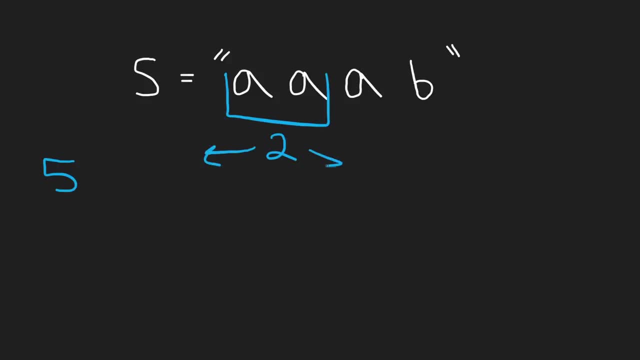 this is a substring of length two, and then we'd expand by one more, So then we'd get a palindrome of length four, And then we'd expand by one more, So then we'd get a palindrome of length two, and et cetera, et cetera. just keep increasing it by two. So this is how we're going to get. 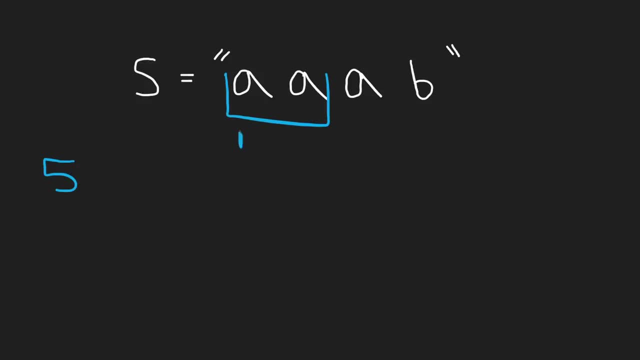 palindromes of even length. So when we do this, we're going to have our left pointer initialized here, And in this case the right pointer is actually just going to be left plus one. before we were doing it as left and right, both starting at the same position. In this case, left, right is. 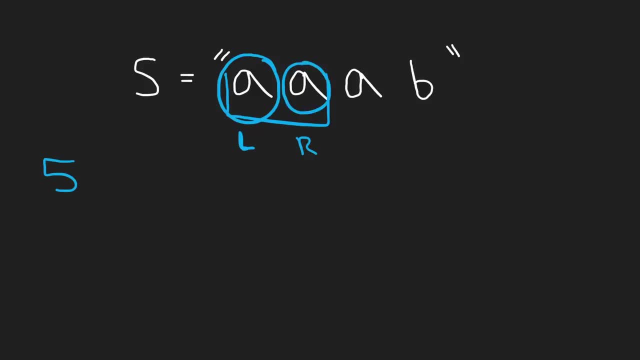 going to be left plus one, And so in this case we see these characters are equal. Therefore they are palindromes. So we can increase our count from five to six. We expand outwards, left and right, but we see left is going to be out of bounds, So then we can stop. So next we're going to 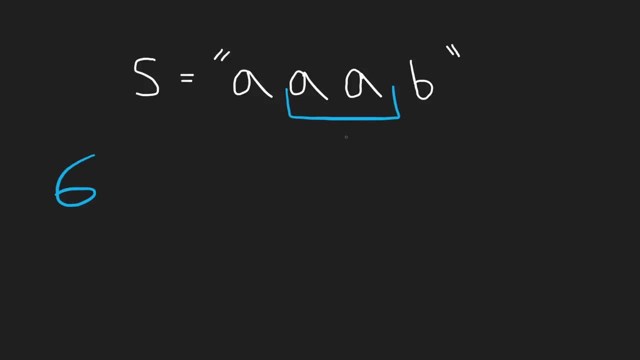 basically do the same thing for every pair of adjacent characters: right to find even length palindromes. So here, left and right are once again the same, So we're going to get our total to be seven. When we expand to the left and right, we see we have an A and we have a B. These 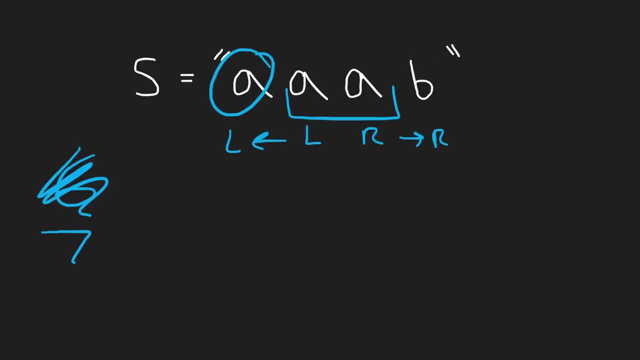 characters are not the same, So we can't continue to expand and we don't increment our result. So now we have seven palindromes- This is the last even length substring that we're going to start at- And the left and right characters are clearly not the same, So we don't continue to expand. 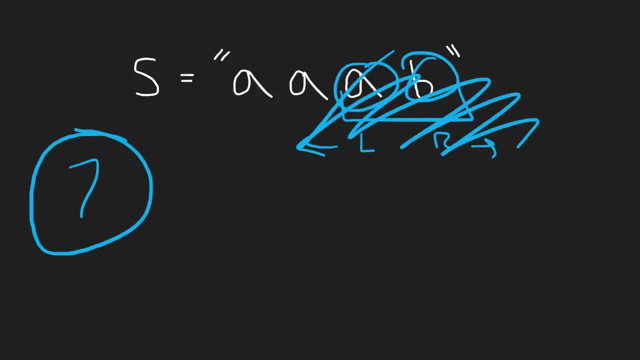 and we don't increment our result. So we're done with everything. here We get a result of seven And the overall time complexity of doing it like this it's going to be big O of N because for, let's say, the odd lengths, palindromes, we're starting at every single position. 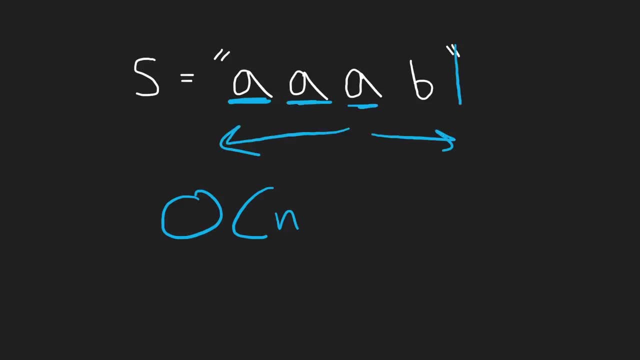 and potentially expanding outwards all the way to the end of the string. So that's going to be an end time operation. So since we're doing it for every single character in the array, it's going to be big O N times N right. So that's basically how we're doing the odd length. 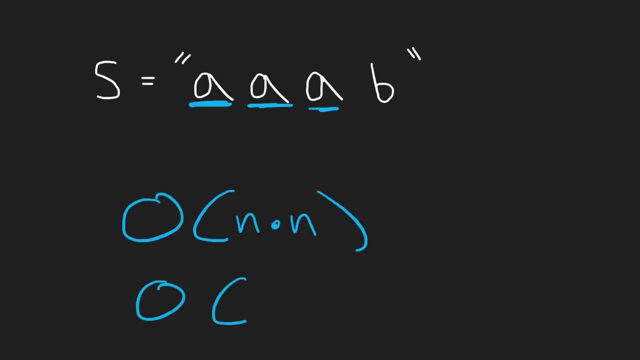 palindromes, And the same time, complexity is going to be true for even length, right? We're basically going through every pair of characters which there are big O of N of them, and then we're still expanding outwards, So that's also going to be big O of N times N. Now, if you add these, 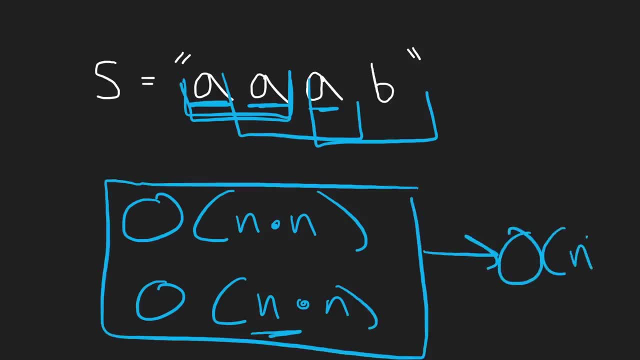 together we're still going to get a overall time complexity of big O N squared. So that's the overall time complexity in this solution, And coding it up is pretty easy, So let's get into that. So let's keep track of a single. 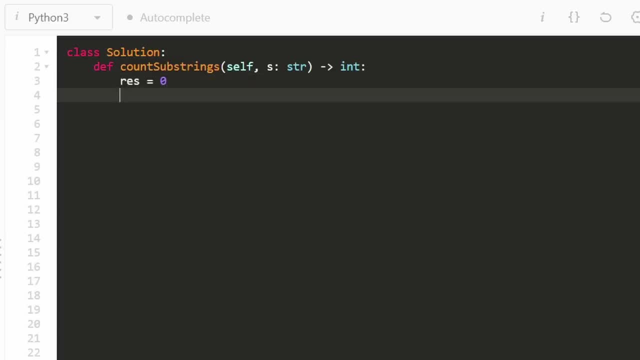 result variable and it's initially going to be zero. It's going to be the count of the palindromic substrings. So we want to go through every single position in the string S and expand from it. right, That's going to give us the odd length palindromes. So we're going to initialize: 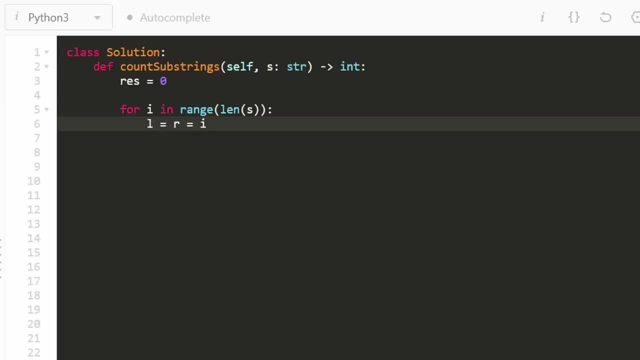 our left and right pointers, both to be set to I, because these are odd length palindromes. And while left is inbound, so while left is greater than or equal to zero and right is inbound, so right is less than the length of the string and the position at left in our string is equal to the position. 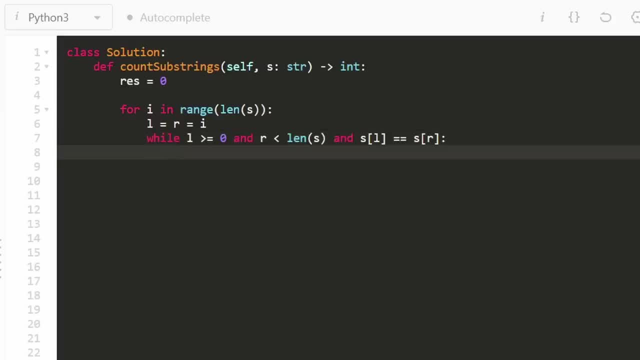 at right in our string. that means we found a palindrome. So let's increment our result by one, Let's shift our left pointer to the left and let's shift our right pointer to the right, And we're going to continue to do that while the pointers are inbounds and the characters are the. 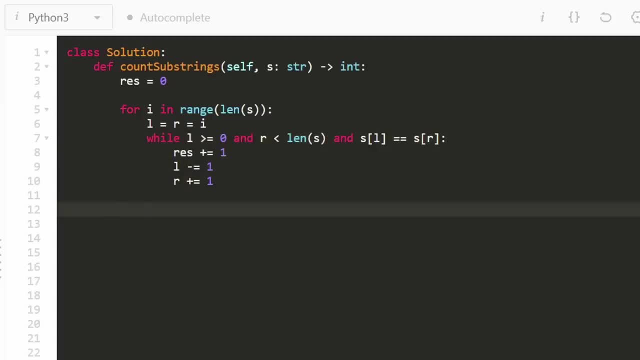 same, Then we're going to continue to increment the number of palindromes, So that's going to give us the palindromes of odd length We can. we don't have to do a separate for loop for the even length palindromes. Let's just do the exact same thing we've done up above. 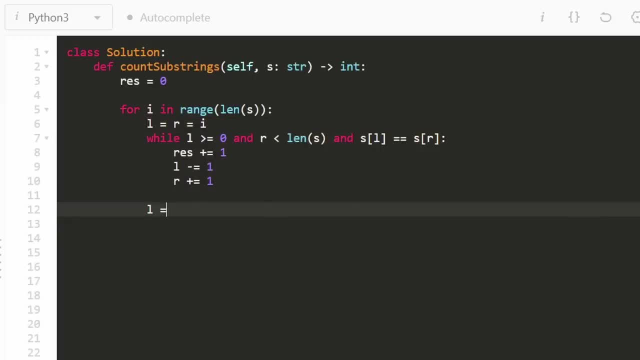 here, except in this case we're going to initialize left to be I, which is what we did before, but we're going to initialize right to be I plus one, which is going to give us the even length palindromes. And once we've done that, we can literally just copy and paste this for loop up. 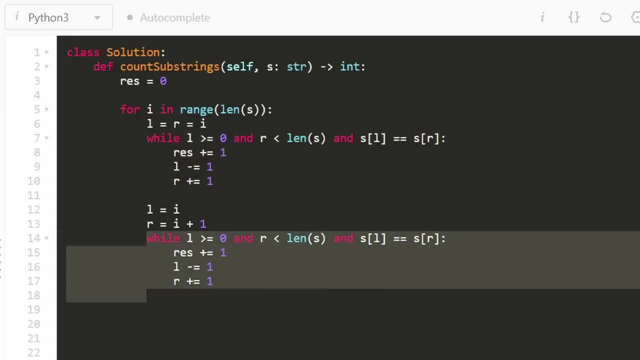 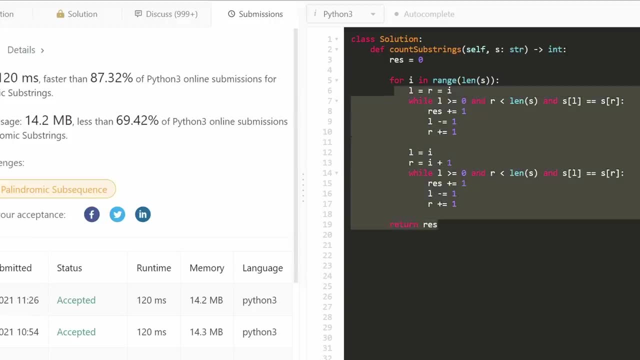 above down here, And then that'll calculate the even length palindromes. So that's going to give us the even length palindromes And then, once that is done, we can go ahead and return our result. Now, as you can see, this solution works. That's the entire thing. It's very efficient. 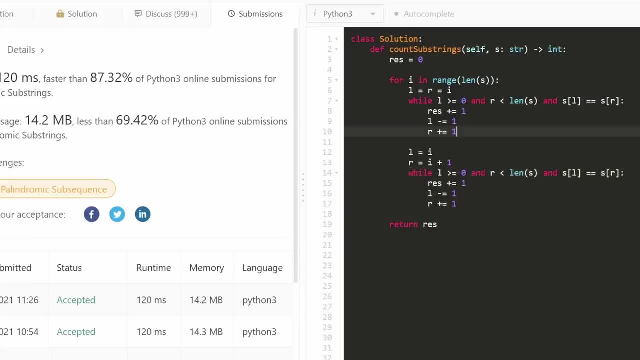 but maybe your interviewer will want you to. you know, this is copy and paste and sometimes they don't like copy and paste. We can basically take these two and condense them down into a single function, So I'm just going to do that, even though I'm sure you could probably figure out. 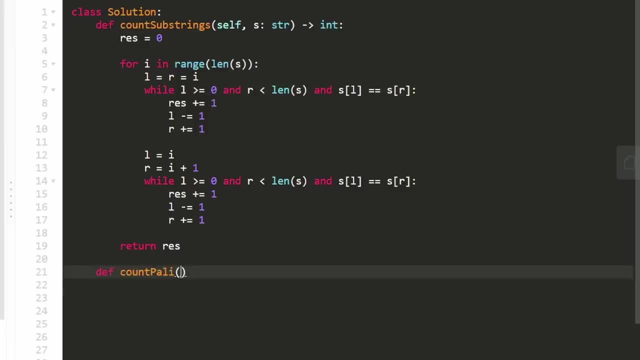 how to do it In this case. it's not too bad. So I'm going to make a function called count palindromes and we'll pass into this the string of the number of palindromes. So I'm going to.